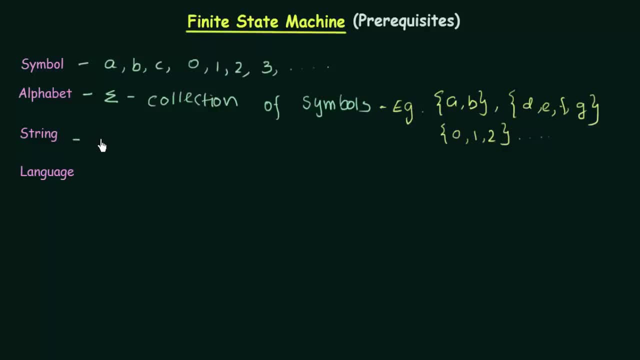 What is a String? A sequence of Symbols is known as String A sequence of Symbols, Strings. actually, it means a sequence of Symbols. Now let's take some examples. Some examples would be like- Let me write it here- A, B just by itself, or 0 by itself, 1 by itself. 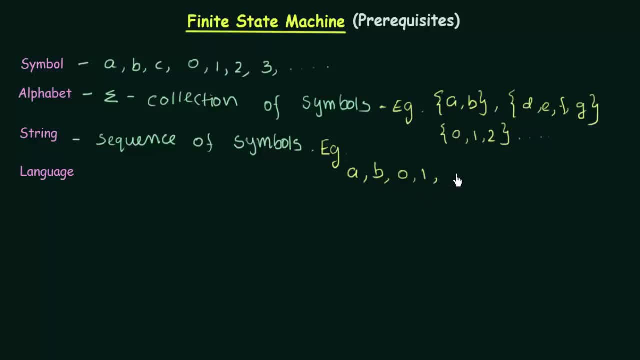 Okay, just by itself. also, we can call it a String. Or we could have other sequences like A A B, B A B or 0,, 1 and so on. Okay, so a sequence of Symbols is known as a String. 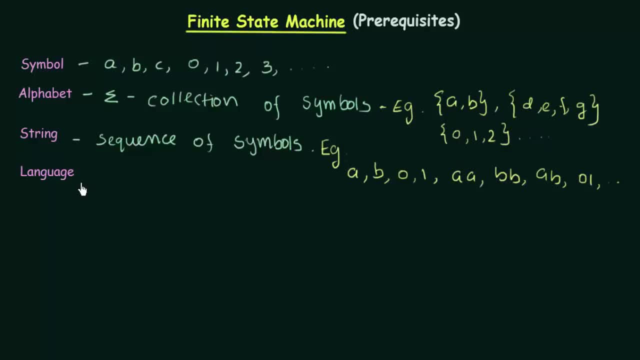 Okay, now let's come to the next one: Language. Now, what is a Language? A Language is actually a set of Strings. A set of Strings- Okay, let me just write it nicely- A set of Strings. A set of Strings is known as a Language. 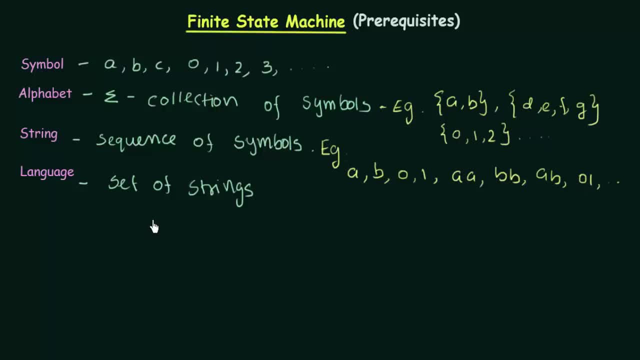 And we can have some example over here. This will become clear with example. Okay, to take an example, Let's say that the alphabet that is here denoted by Sigma, The alphabet that I have, is the two digits 0 and 1.. 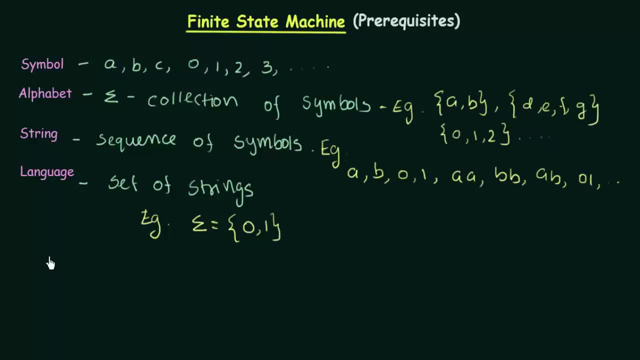 0 and 1 are my alphabets, And now let's try to define some languages over these alphabets 0, 1.. So let me say I have language L1.. Which is the set of Strings, The set of all Strings of length 2.. 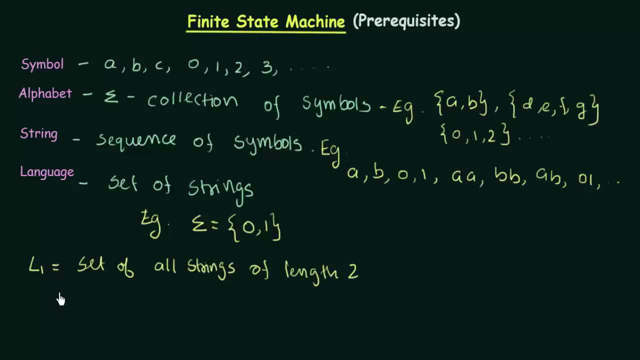 The set of all Strings of length 2.. So what would they be? They would be: my alphabets are 0 and 1.. So what would be the set of all Strings of length 2 over 0, 1?? 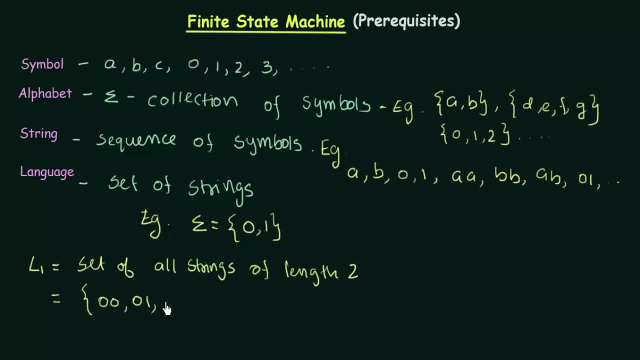 0, 0, 0, 1, 1, 0 and 1, 1.. So these are the set of all Strings of length 2 over the alphabets 0 and 1.. Now let's take another example. 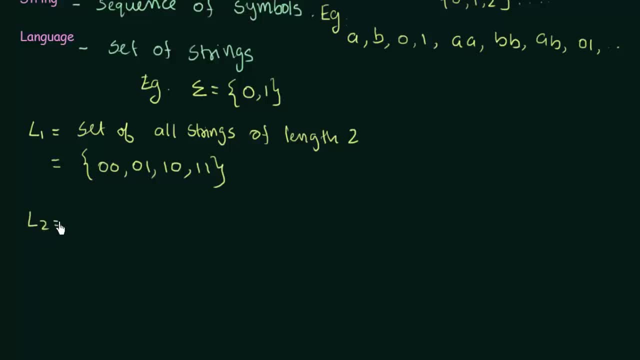 L2.. Now, L2 is the set of all Strings of length 3.. Set of all Strings of length 3.. Now, what would these be? My alphabets are 0 and 1.. So what would be the set of all Strings of length 3?? 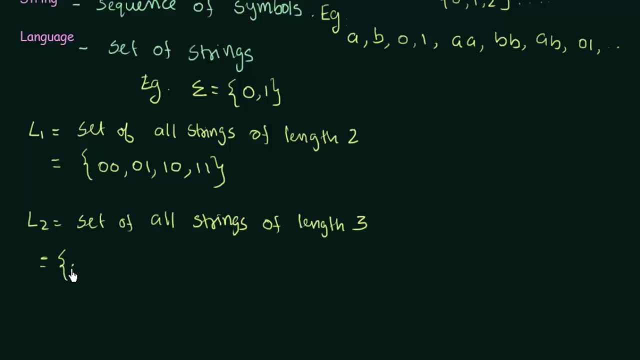 I guess you have already thought about it: 0, 0, 0, 0, 0, 1, 0, 1, 0, 0, 1, 1, 1, 0, 0, 1, 0, 1. 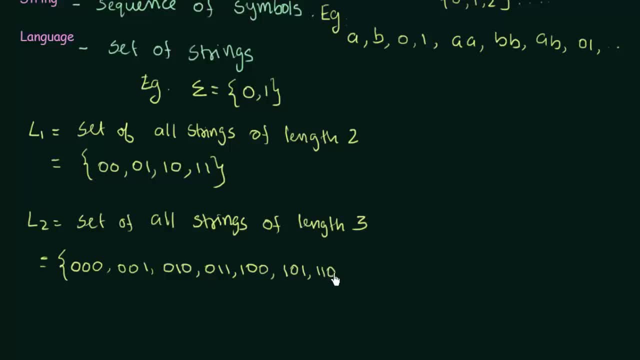 and 1, 1, 0 and 1, 1, 1.. So these are the set of all Strings of length 3 over the alphabets 0 and 1.. Now let me take another example over here. 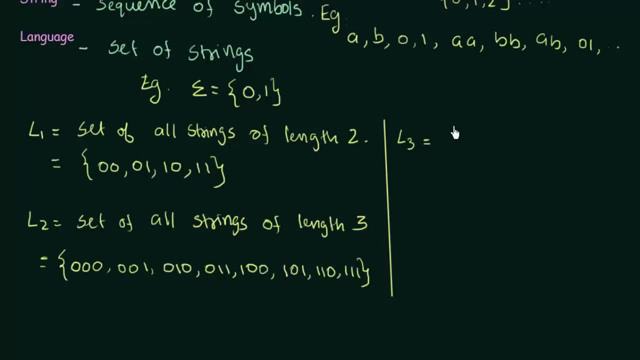 Which will be L3.. L3 will be the set of all Strings of. Okay, let us say that it is the set of all Strings that begin with 0.. The set of all Strings which begins with 0 is L3.. 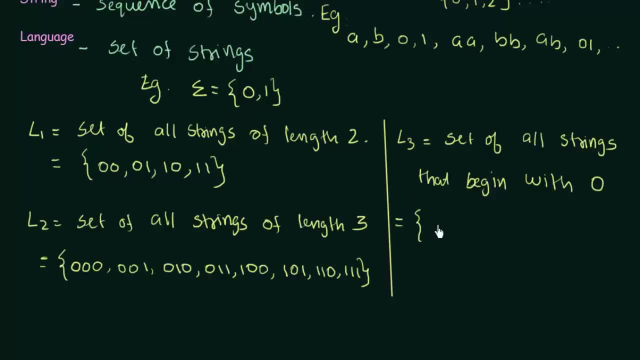 So my alphabet sets are still 0 and 1.. So what would they be? They would be like 0, 0, 0, 0, 1, 0, 0, 0, 0, 0, 0, 1. 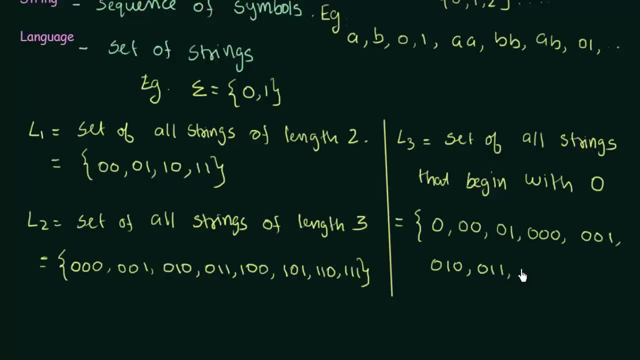 0, 1, 0, 1, 1 and 0, 0, 0, 0, and it goes on. this is actually an infinite set. so the two example that we took here, l1 and l2, these two l, l1 and l2, they are finite. 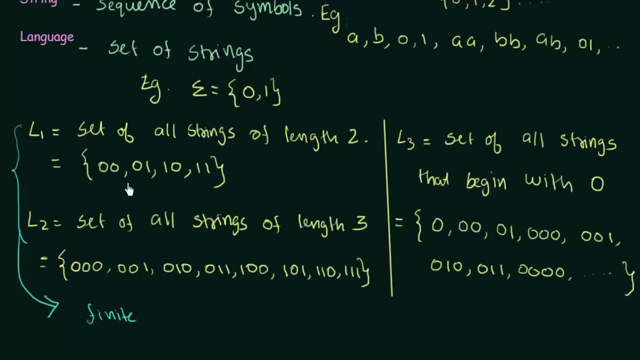 sets. they are finite sets. why? because they have finite number of elements. here we have four elements, here we had eight elements, but this l3- l3- is a infinite set, it is an infinite language. why? because this goes on, this does not end. there are infinite number of elements in this set. so I think, by taking these, 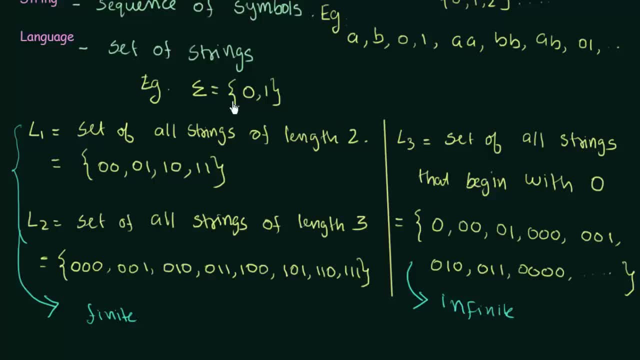 examples l1, l2 and l3. over these alphabets 0 and 1, the concept of language became clear to us. so language are a set of strings over some alphabets. you okay. so I hope that was clear now. the next thing that we need to discuss is: 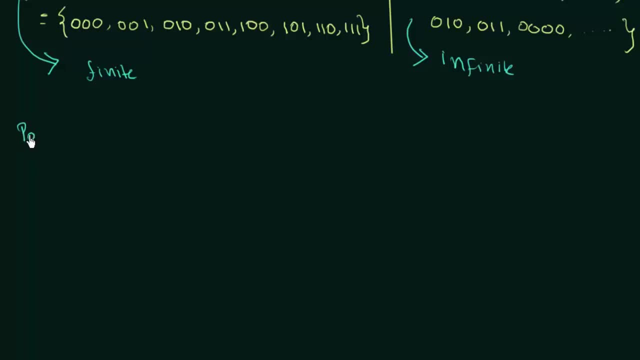 known as powers of Sigma. powers of Sigma. so this is the next thing that we will be discussing. okay, now to demonstrate this, let me take an example again. suppose my alphabet set is again 0-1, my alphabet Sigma is 1. now I'm going to define the powers of Sigma. so 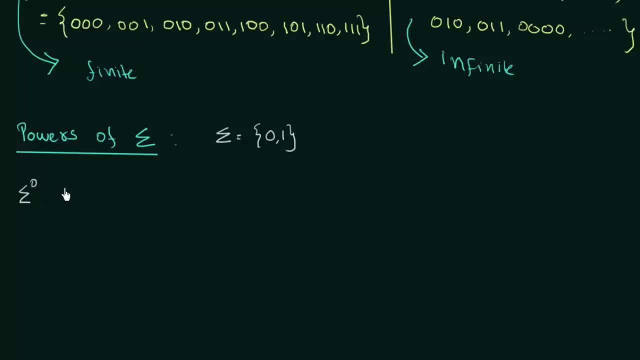 first of all, I mean defined Sigma power-0. now, what is Sigma power-0? Sigma power-0 with the set of all strings of length zero. this is equal to the set of all strings of length of length 0, 0. length 0: 0. now, what would this be? I would be. I would denote this using Sigma power 0. 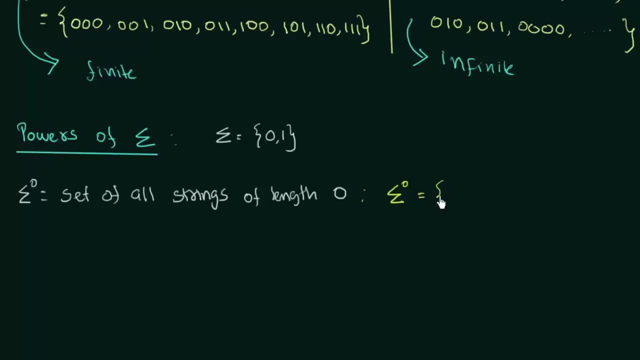 and this is denoted by a special symbol called epsilon. this epsilon is used to denote the set of all strings of length 0 denoted by Sigma power 0. so remember that epsilon means it is a set of all strings of length 0. okay, so that was. 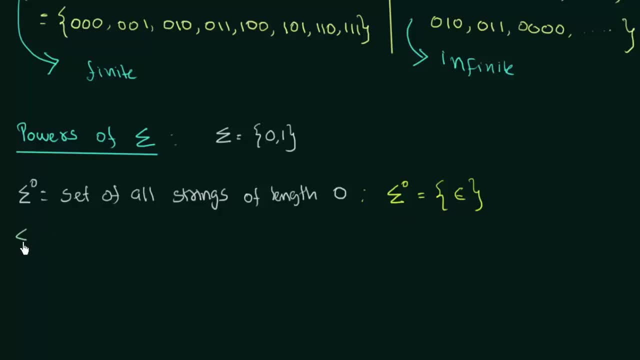 about a set of all strings of length 0. now let us come to the next one, Sigma power 1. I think you have already guessed what it is. Sigma power 1 is a set of all strings of length 1. now what would that be? that is, 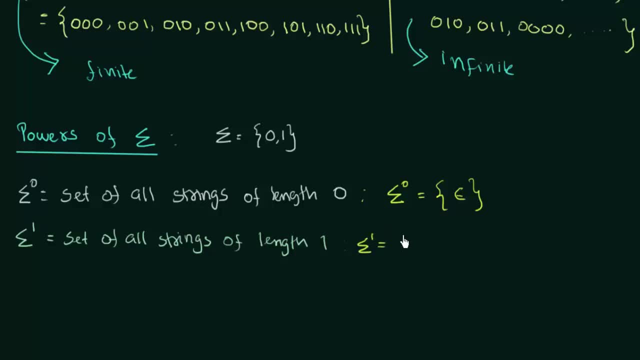 Sigma power 1 is equal to what? would that be 0 and 1? the set of all strings of length 1 are 0 and 1, here 0. the length of this is just 1 and the length of this one is also just 1. so the all the set of strings of length 1 is Sigma. 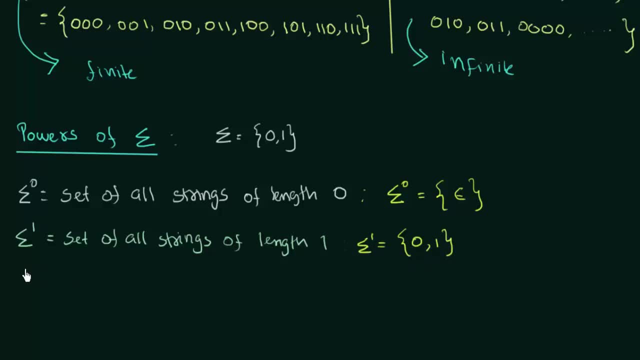 power 1. okay, so the next one is Sigma power 2, which is a set of all strings of length 2. so what would they be? Sigma power 2? I hope you have already guessed it. they are 0, 0, 0, 1, 1, 0 and 1, 1. these are the set of all strings. 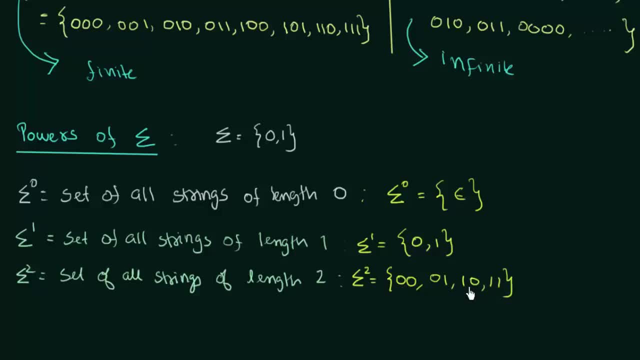 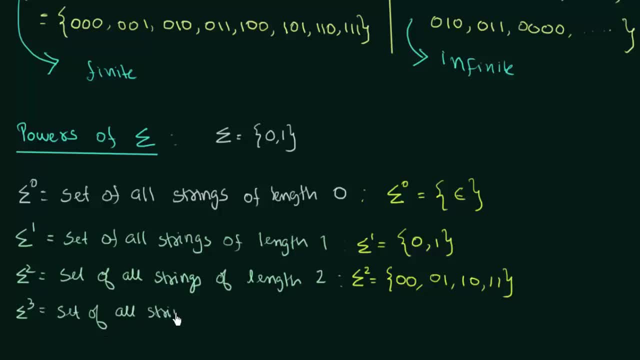 set of all strings of length 3. okay, so what would they be? I know you must have guessed it: they are 0, 0, 0, 0, 1 0, 1 0, 0, 1, 1, 1, 0, 0, 1 0, 1, 1, 1 0 and 1 1 1. so these are the set of all strings of length 3. see, there are. 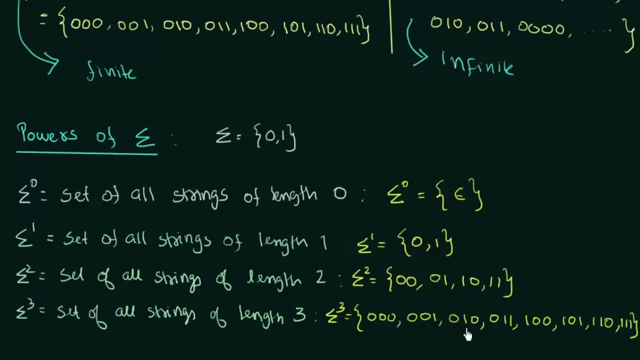 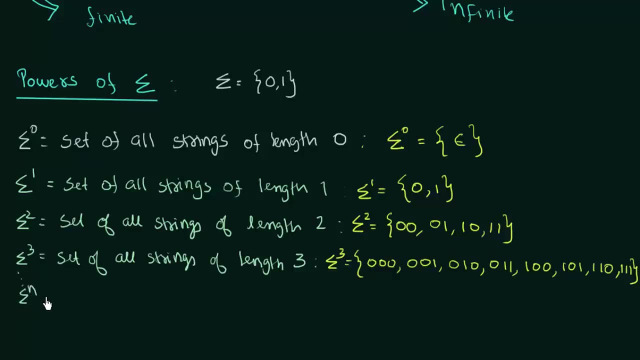 3, 1, 2, 3, 1, 2, 3, 1, 2, 3, and so on. so these are all the sets of strings of length 3, denoted by sigma power 3, and then it goes on like that, and then it comes to Sigma power n. Sigma power n is the. 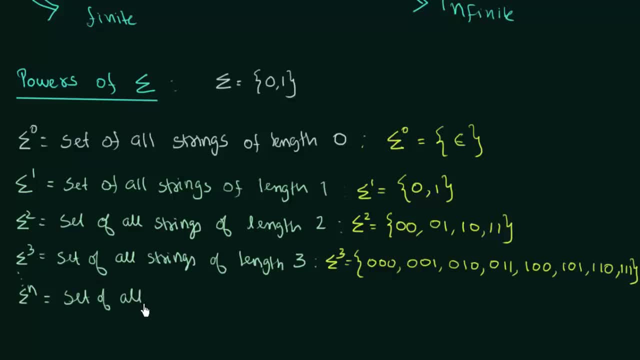 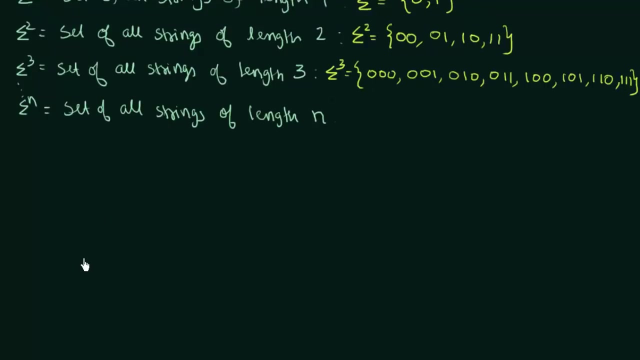 set of all strings of length. what would be the length? what would be the length? the length would be n. Sigma power: n would be the set of all strings of length, n. okay, so that was about the powers of n. sigma, sigma power: 1, 2, 3 up to n. so the next term that we need to discuss is known as cardinality. 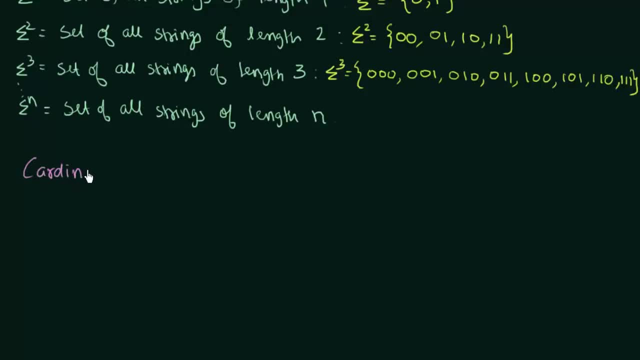 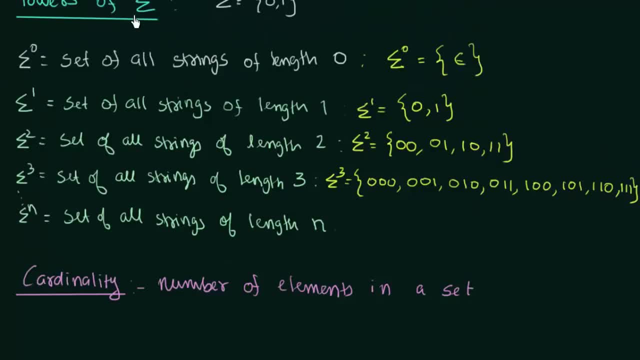 set. this is known as cardinality. so let set this is known as cardinality. so let us quickly check what are the cardinality. us quickly check what are the cardinality. us quickly check what are the cardinality of these powers of Sigma. so, sigma power 0. 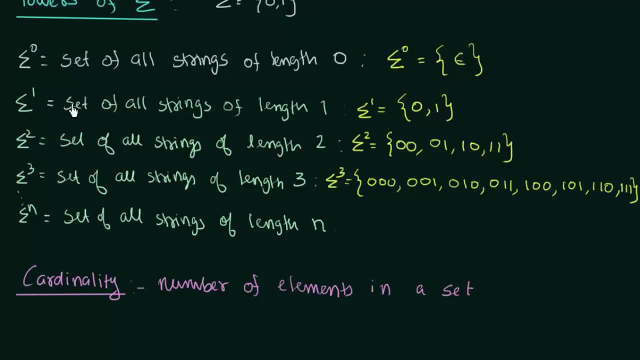 of these powers of Sigma, so sigma power 0 of these powers of Sigma, so sigma power 0 has only one element. so the cardinality has only one element. so the cardinality has only one element. so the cardinality is 1, and in Sigma power 1 there are two. 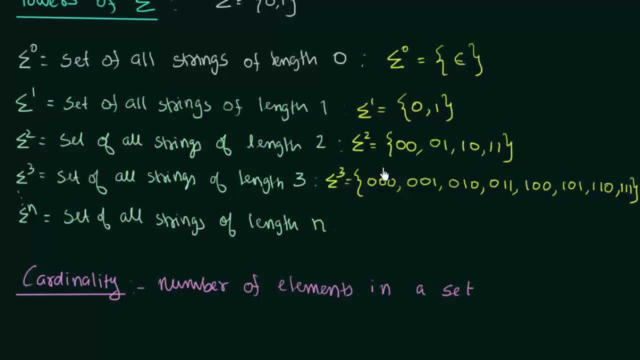 is 1 and in Sigma power 1 there are two- is 1 and in Sigma power 1 there are two: elements- 1- 2, so the cardinality is 2 and elements 1- 2, so the cardinality is 2 and And for sigma power 2, it is 4.. 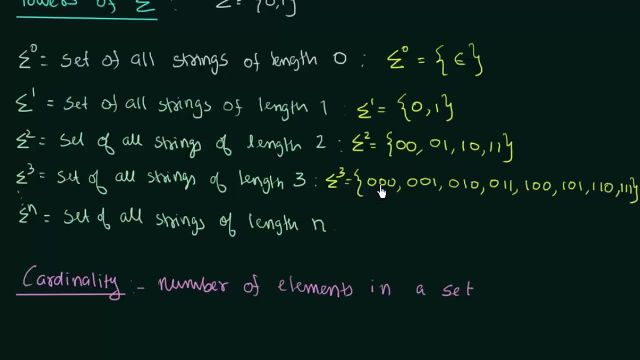 1,, 2,, 3,, 4.. And for sigma power 3, it is 1,, 2,, 3,, 4,, 5,, 6,, 7,, 8.. The cardinality is 8.. 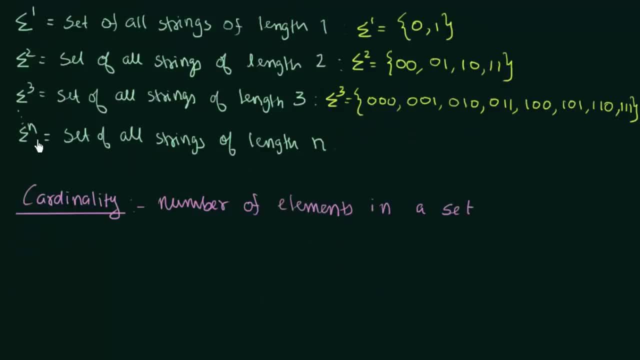 And what about sigma power n? In sigma power n it is a set of all strings of length n. So what would be the cardinality? The cardinality of sigma power n would be 2 power n. So this is the formula that is followed for the cardinality. 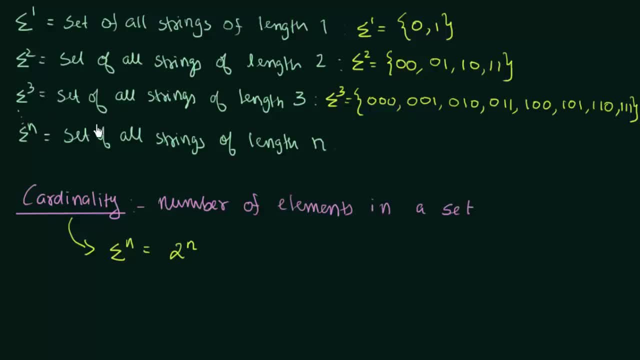 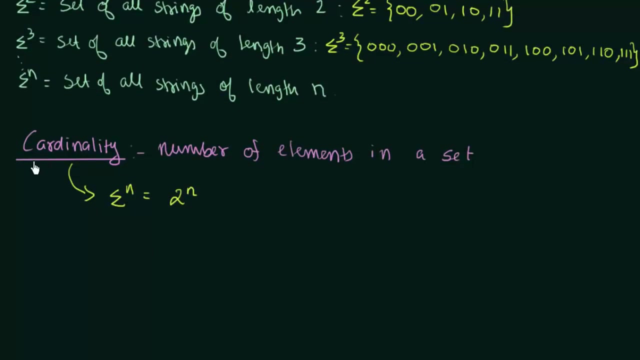 If the alphabet is over two digits, just 0 and 1.. So for sigma power n, the cardinality is 2 power n. Okay, So let's come to the last term that we need to discuss, That is, sigma star. 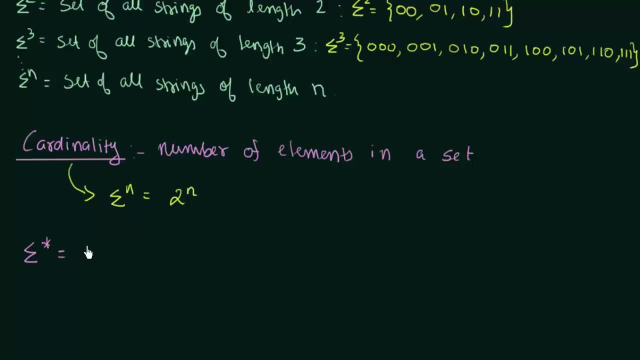 Sigma star. So in this sigma star the star can be replaced with sigma power 0, union sigma power 1, union sigma power 2, union sigma power 3, and so on It goes on. So let us put the values here and see what would we get.